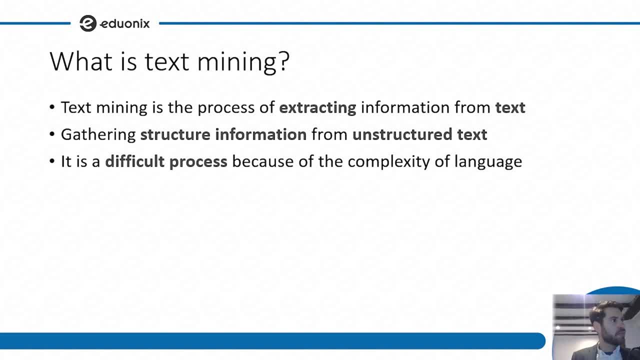 Think of all the punctuations that we have, the comas, the complexity of the language. So all that extractor information. we want to put it in somehow in an extractor way. We're going to see it is a difficult process because of language, you know. 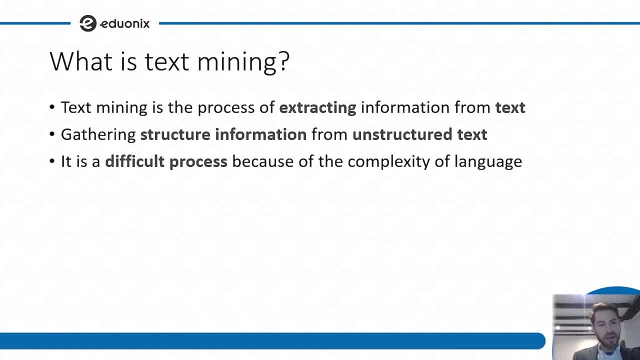 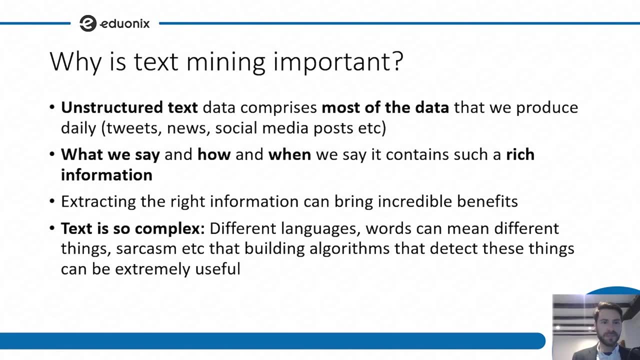 characterizes, you know, our thoughts, our ideas. It characterizes also our mood, our sarcasm. So we're going to see that It's quite, quite difficult. Why is it important? Well, most of the data that we produce daily comes actually from text. 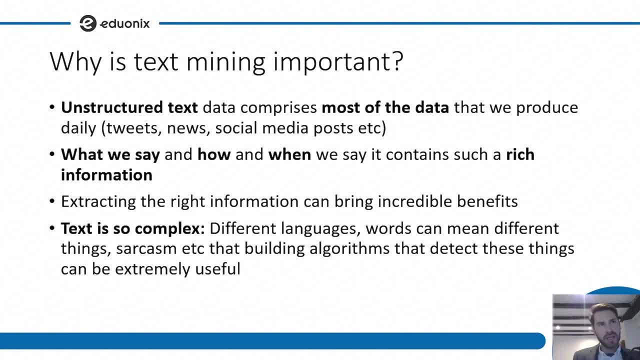 We have tweets, we have news, we have social media posts and data. we know is power or information. is power The information that we have nowadays of, for example, the stock market or the economy, or how we feel we're expressing all this throughout text? 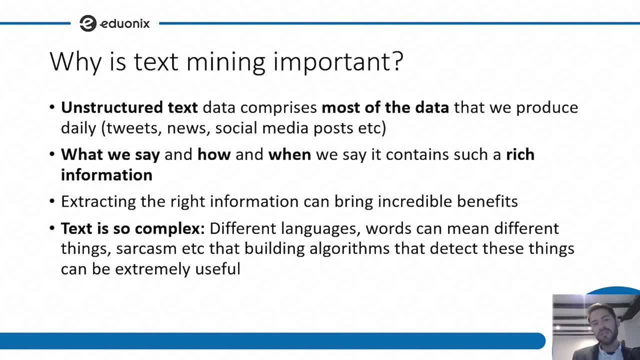 And having this information on, able to cover this information is quite important. So what we say, how and when we say, it contains a lot of rich information, From our mood to the way we feel or the way we think into the future. 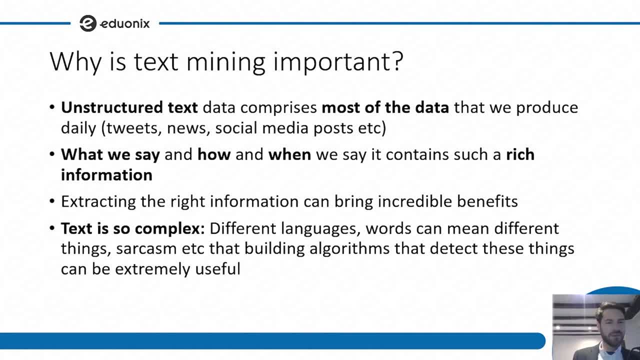 But text is really, really complex. We have different languages, Words can mean different things, We have sarcasm that we can think It contains a lot of information, It contains something positive, but it doesn't. And using exactly the same words, 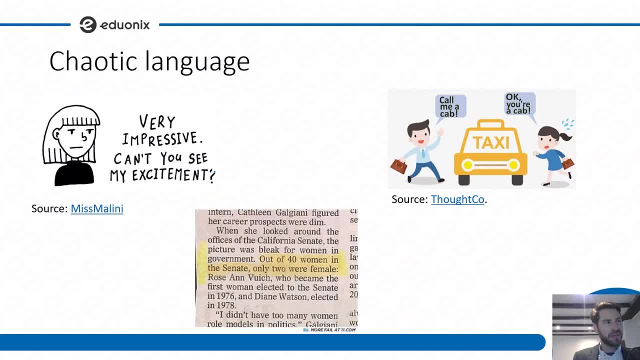 So to give you a little bit of information, you know of why text mining is important. let's just go through these three examples. The first one, this girl says very impressive. Can you see my excitement If you look at the words impressive excitement. it contains a positive mood, right? 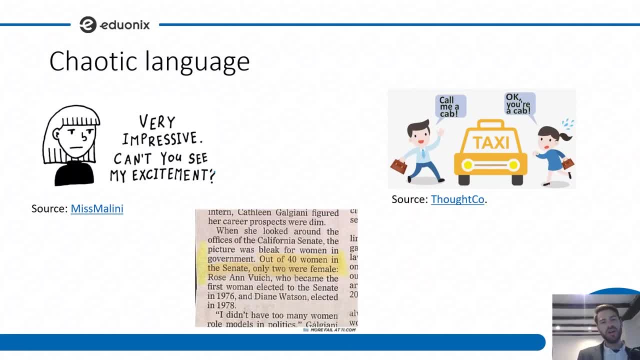 But nonetheless she's being sarcastic. She means just the opposite. So even though you could use these exactly the same words to describe something really positive, like impressive, you are meaning exactly the opposite. In this other example we see a guy saying: call me a cab. 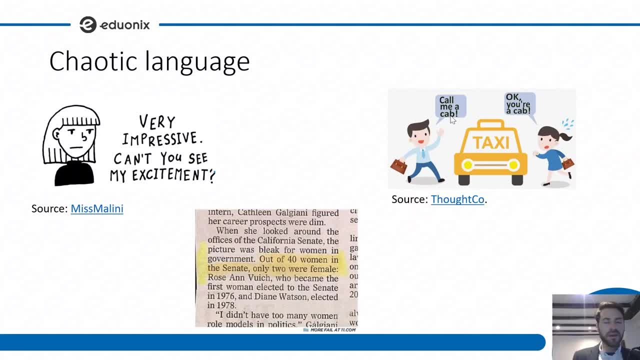 And the girl replies: okay, you're a cab. So here we see how, once again, you know, based on the language, how it's built, it can contain different meaning, right? Clearly, the gentleman here wants to get a taxi, but the girl is just valid. 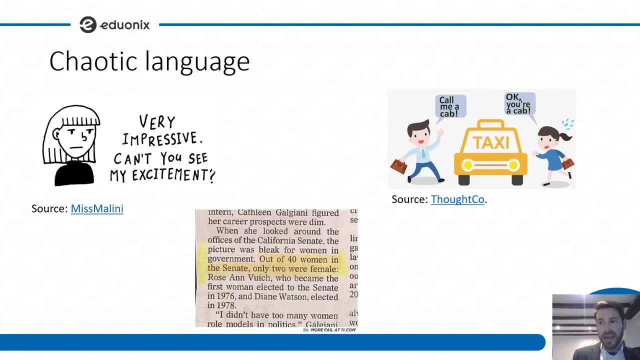 They say: okay, if you want me to call you a cab, I'm going to call you a cab, You are a cab. And also we have sometimes- you know that- mistakes in our writing. For example, if we see this piece of news, out of 40 women in the Senate, only two were female. 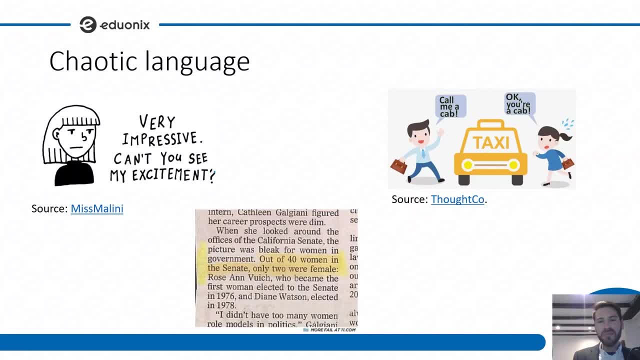 Okay. So sometimes what we mean, you know, is not properly written, contains some mistakes. especially in this era, where things tend to be a little bit faster, It's a little bit difficult, you know, to use the right words. 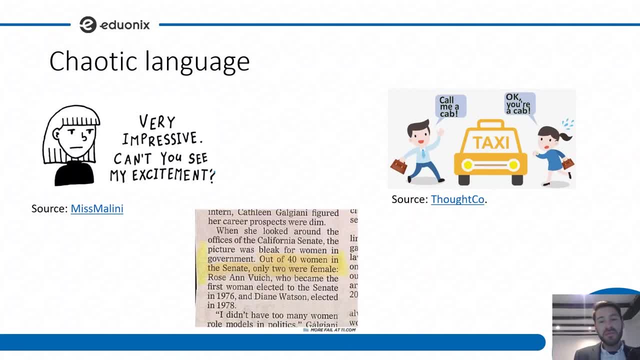 So the message might not be so clear or it might be a little bit ambiguous, right? So just with these examples, I just want you to open your mind to see the complexity of the language per se, And this is just in English. 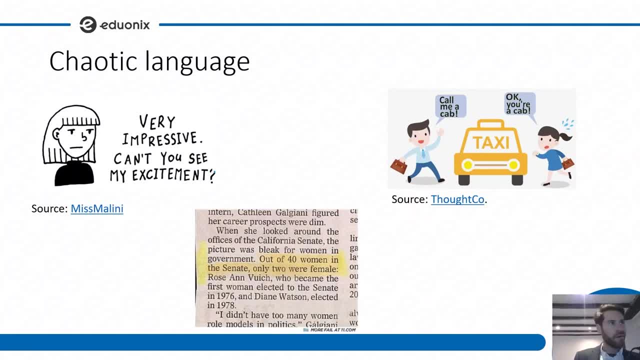 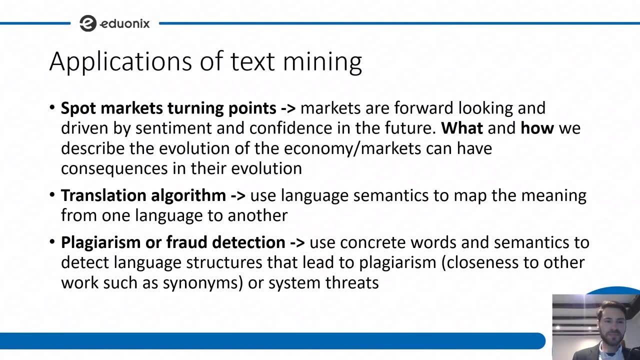 Imagine, you know, we have a wide range of languages where the future, the past or something is composed from different wordings. Some applications that I particularly find fascinating on the text mining field. what it can be used for is, for example, spot market turning points. 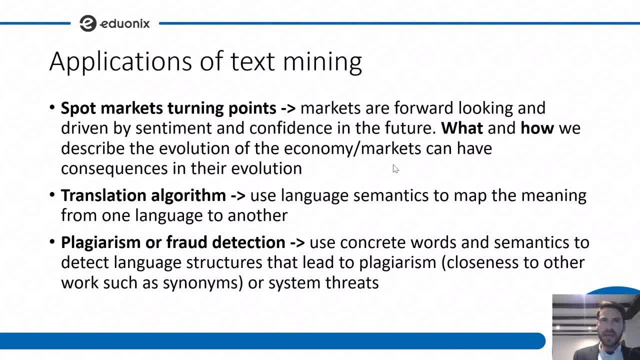 I've been doing that throughout my research And the argument is the following: Markets are falling. People were looking and driven by sentiment and confident in the future. So imagine you know some respectable individual that knows a lot about finance states that markets are going to collapse tomorrow. 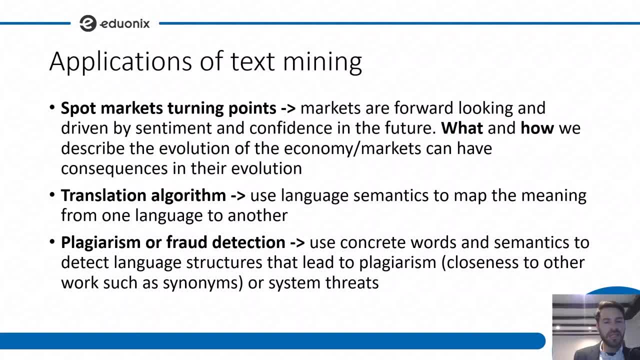 This message that can be conveyed in news or in media is going to drive fear to the individuals. The words that this person uses, how it phrases and how it is composed is going to is going to drive the fear on the people. that ultimately can have consequences in the economy. 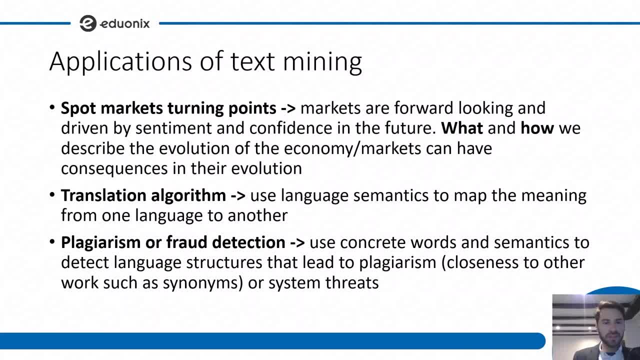 Also, a lot of the research or a lot of the applications of text mining are translation algorithms. They use language semantics. So different languages they have, as we will see throughout this course. they have different semantics, They have different relationships among words. 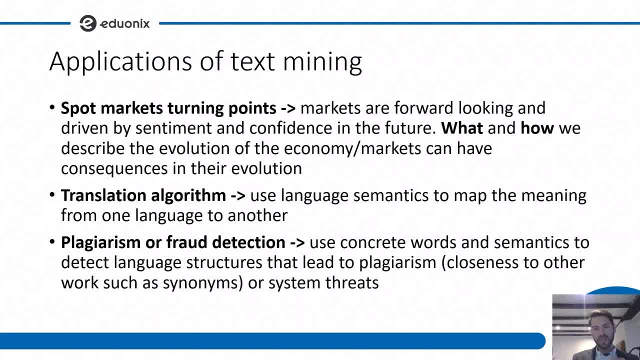 And what these algorithms are doing is they're mapping one meaning to another. Of course, the mapping is a little bit complex because of the complexity of the of the different languages that we have. Some languages are more prone on using adverbs, you know, to describe certain situations. 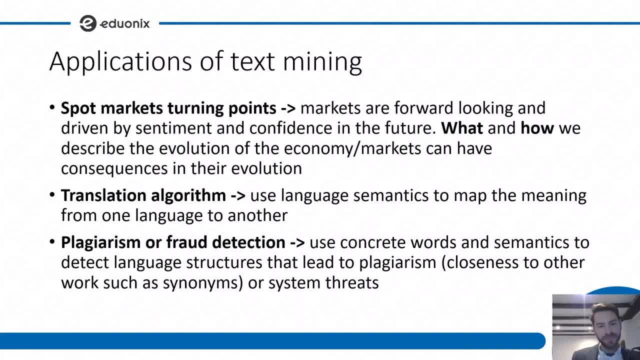 Other languages are more prone on using verbs, for example. Also, a lot of algorithms that are used in text mining are more prone on using verbs. So a lot of algorithms that we see nowadays can be used for plagiarism or fraud detection. So these algorithms, they would use concrete words and semantics to detect language structures that have led to plagiarism. 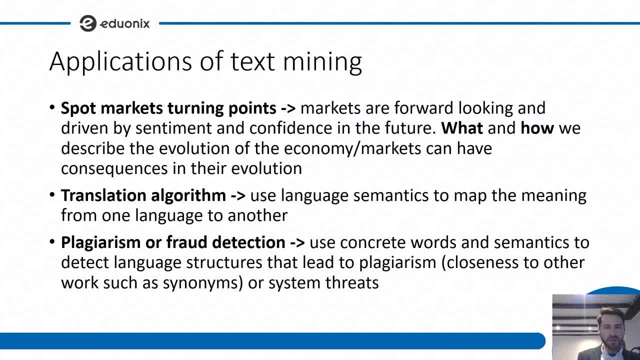 Imagine you know you're plagiarizing some work. You are going to try to use synonyms. You are not going to do a copy and paste, but you might use synonyms. Based on this structure, the algorithm can consequently say that the matching between these two sentences are really really exact or are really almost equal to one. 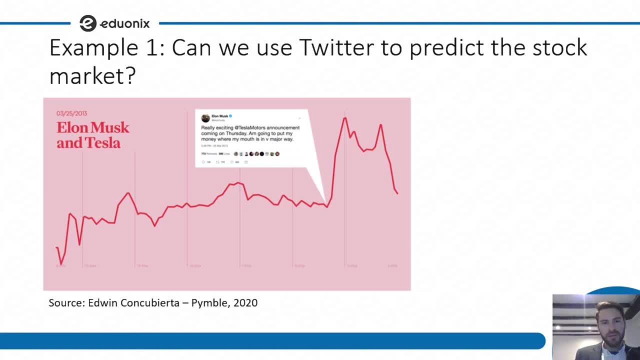 Let me put a few more examples on how text mining is useful and why it's useful. In example one, this is some research that tries to assess, you know, to what extent Twitter can predict the stock market. Here we see a tweet done by Elon Musk that says: really exciting Tesla Motors. 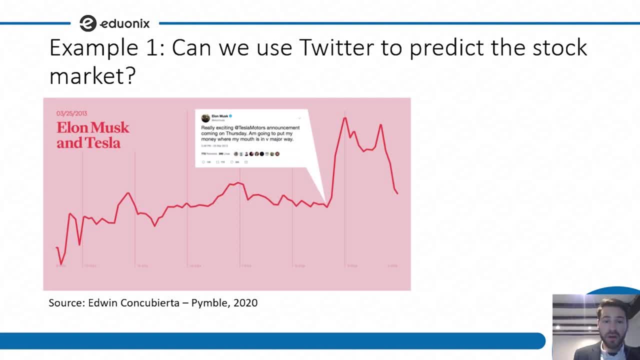 announcement coming on Thursday: I'm going to put my money where my mouth is in the major way. Now the message is: somehow it's not so straightforward. Okay, So he says that he's gonna put his, he's probably gonna invest a little bit more. 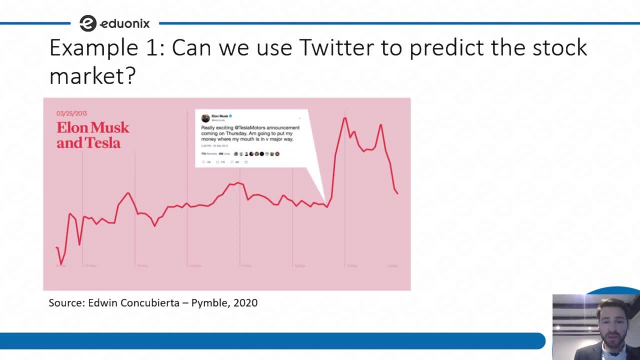 but he's not referring, you know to, to the exact word investment. he says: i'm going to put my money where my mouth is. that is something that means in english: i'm going to, i'm going to set what i, i'm going to do what i said, but maybe in other languages means something different. 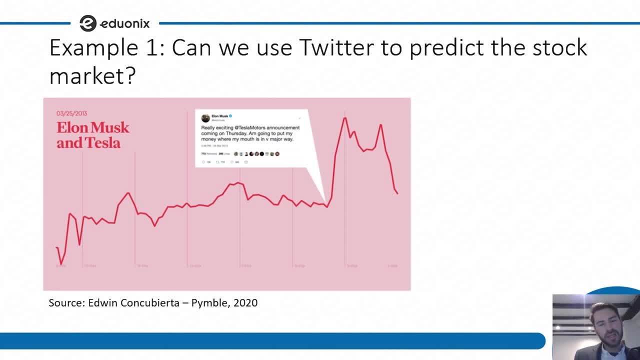 so, as you can see, for that, for any automatized algorithm, it's going to be really hard to detect this language, to detect these patterns. nonetheless, the human brain understands this message and prompts the stock market to to rise and to go up. people expect some actions. people expect. 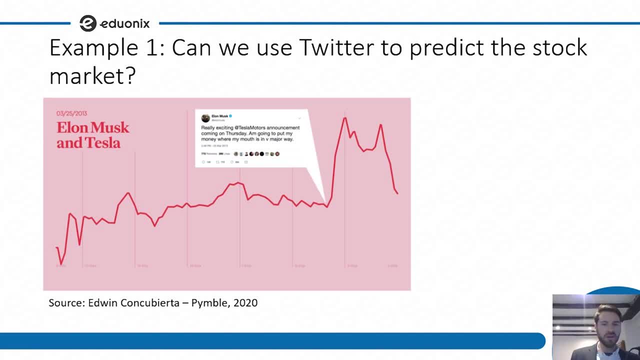 that something major is going to happen, that this guy is probably going to invest in tesla and therefore maybe it's a good opportunity. now we don't know what came later on- if there were some following tweets or something. we know that from this graph that they came back. but the interesting point is that right after 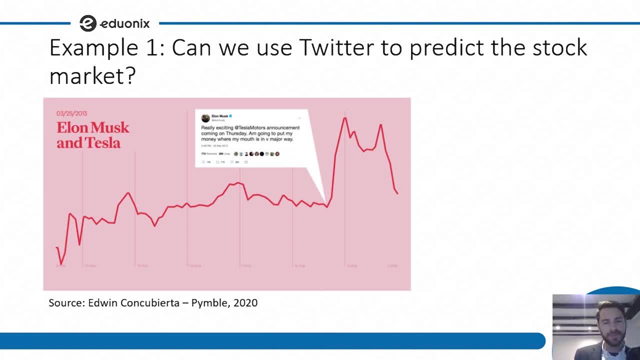 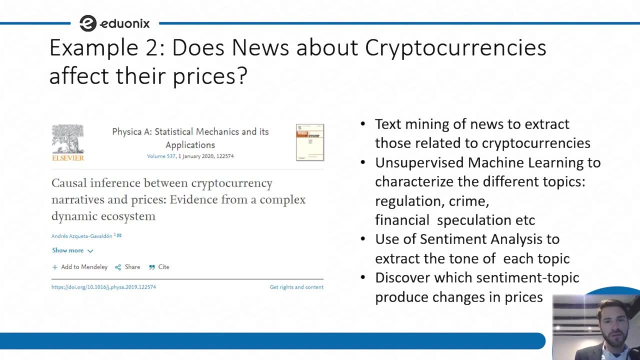 elon musk mentioned this tweet. the stock market jumped in an example and this is from a. this comes from my particular research. different example is here. i try to assess whether or not cryptocurrencies affect news about cryptocurrencies affect their prices and in order to do that, i was 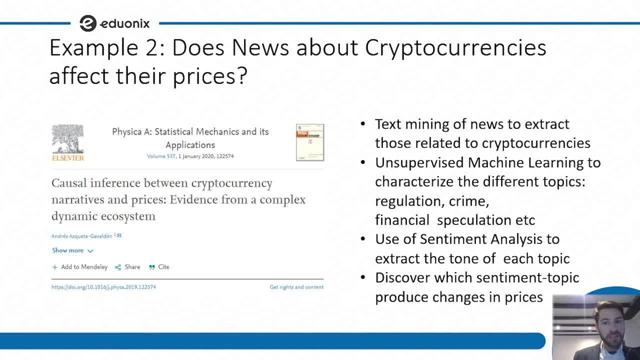 extracting news that they were characterizing or they were describing the crypto, cryptocurrencies and i was using some unsupervised machine learning algorithms that were going to come through it. so i acknowledge that you know, not all news describing cryptocurrencies. they're equal. they were. they were the same in the sense that they would convey the same message. 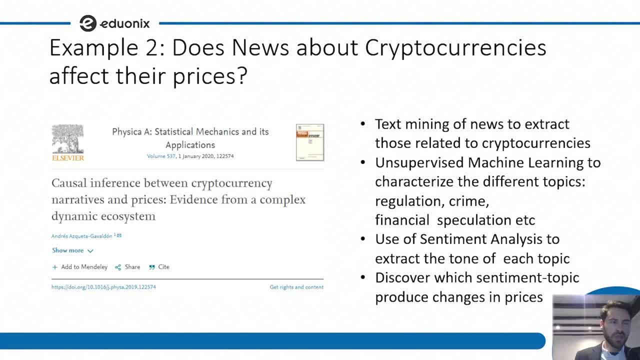 so that's why i had to encourage an unsupervised algorithm in order to check the different themes and the different perspectives, to understand the different topics that they were. around this, moreover, i acknowledged that the sentiment was also important, and let me get back. using the unsupervised machine learning algorithm, i was able to characterize different topics for 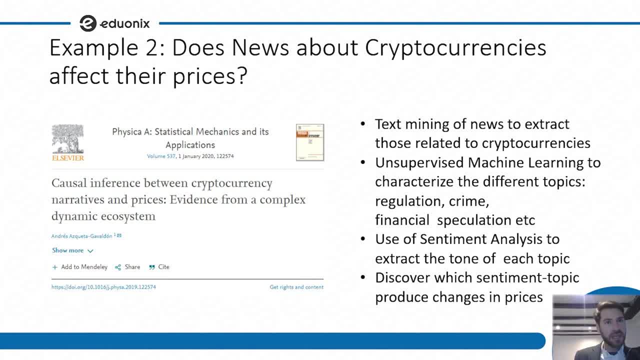 example based on regulation, crime, financial speculation, etc. later on i match it to to the sentiment analysis, to the sentiment that this, these different topics had and ultimately, i assess the relationship we try with with prices. i observe how negative, negative news, for example regarding crime, drove the prices down and also how 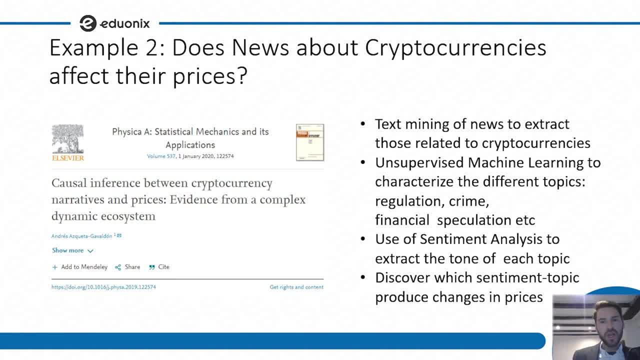 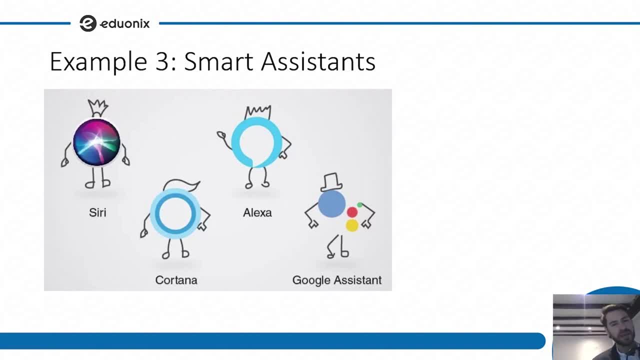 positive news regarding, you know, financial speculation drove cryptocurrencies up in a different example. our last example. we all, we all- have seen smart assistants: siri cortana, alexa, google assistant. they all use capable and really sophisticated algorithms to detect. what do you mean when you're asking something? you can ask any questions. you can ask. 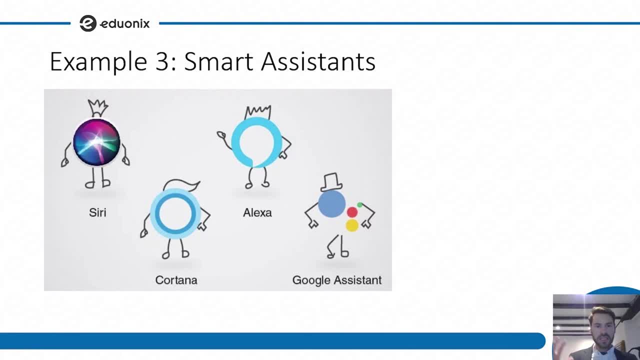 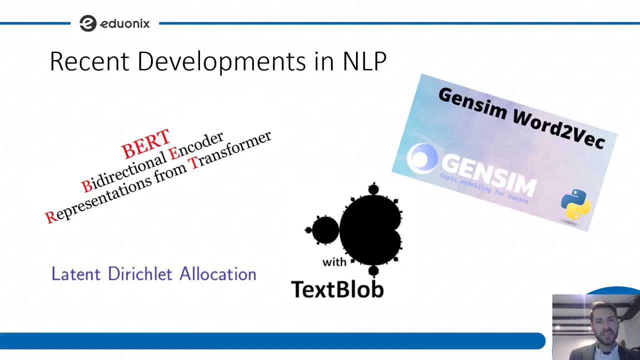 you know reminders, so these assistants, they really have a really powerful mapping of the, of the language, of all the things that that you can imagine, of the complexity of the, of the, of the wording that you might use these algorithms they can assist you with. so recent developments in. 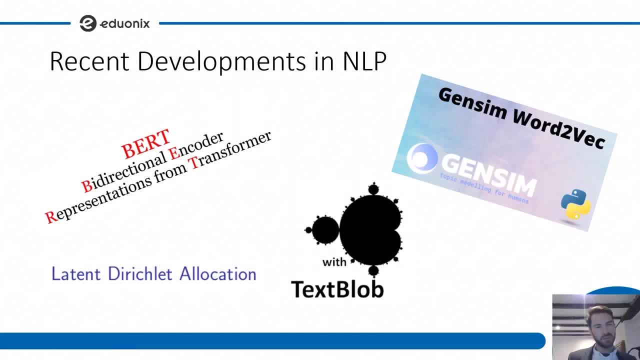 natural language processing, where it has been an explosion on it recently, the one of the most state-of-the-art- you know the- by the time i'm releasing this video- is bird, a bi-directional encoder, representation from transformers, really capable of assessing the structure of the language, of composing, of assessing, you know to what extent. 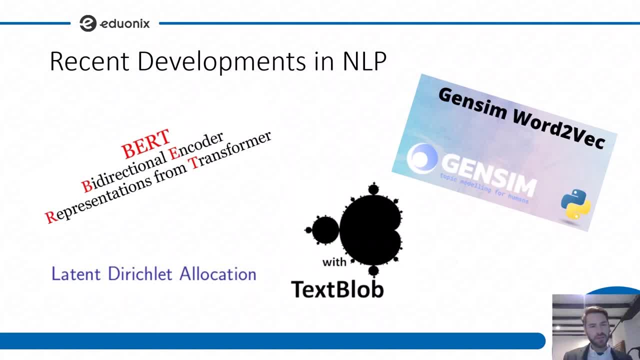 this word has a meaning on. this other word, as we're going to see later on, later in this later location, allows, you know, to build topics, to develop semantics in an unsupervised way, throughout, throughout, any corpus or composition of documents. text blob is really, really powerful for. 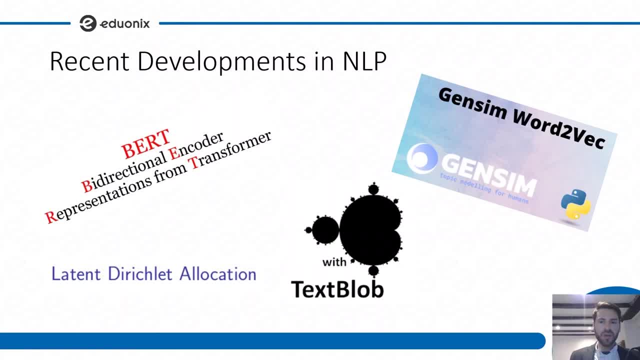 for us. assessing the, the sentiment in sentences or documents and dancing word to back also has been used to analyze the semantics. now that we have seen the complexities of the language in the form of examples and we have highlighted, for example, the complexities of them, how, like the different words can have, like different meanings, how, 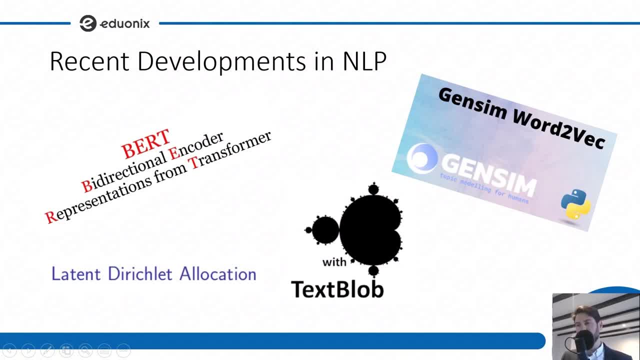 depending on the context you know like or might have a different meaning now, in this say, what we're going to talk about a keyword extraction, and we're going to also offer an illustration of it using the google trends. keywords extraction as sales we're going to see is the most basic. 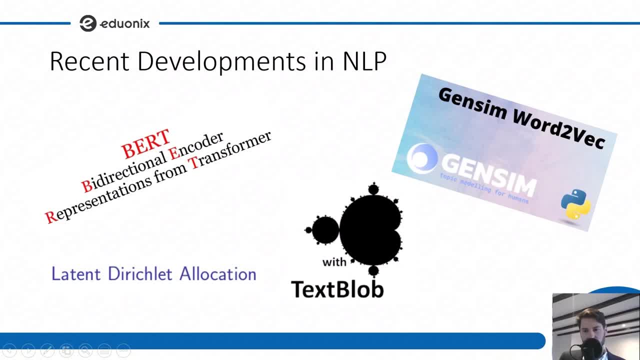 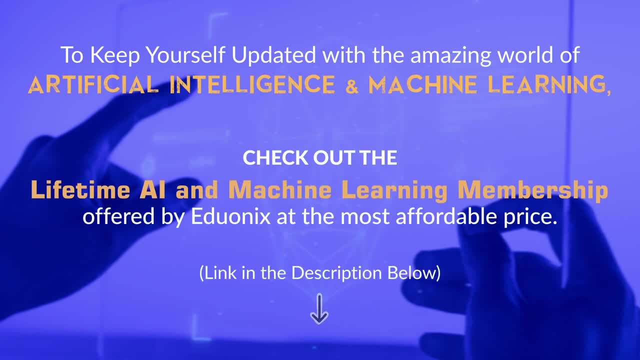 form of a natural language processing, but nonetheless it's going to be quite a useful one.